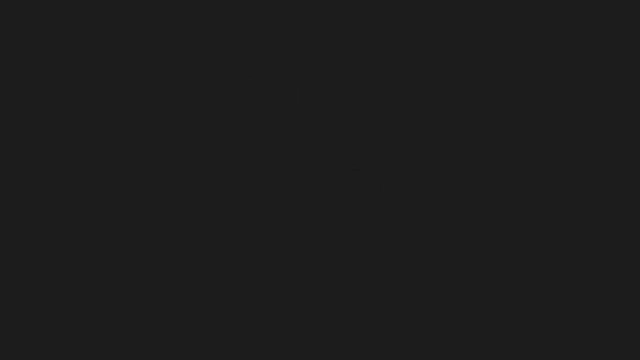 Formally, a linear functional is any linear map L that goes from the vector space to a scalar number, which may be real or complex. Basically, it's any linear map that takes in a vector and spits out a number. Now that we know what a linear functional is, let's move back to R2 and figure out what 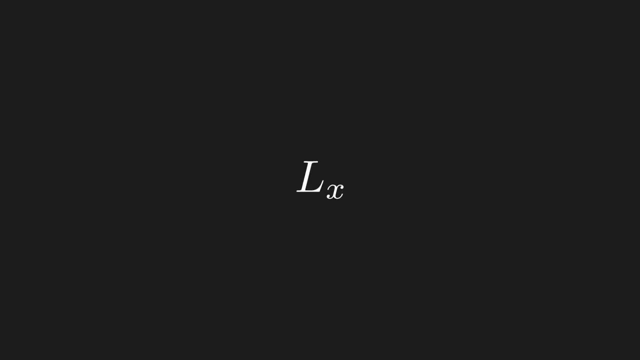 the matrix for LX looks like. I encourage you to try it out on your own before we run through it. Now, that being said, we know that LX takes us from 2 dimensions down to 1 dimension, So we know we have a 1 by 2 matrix. 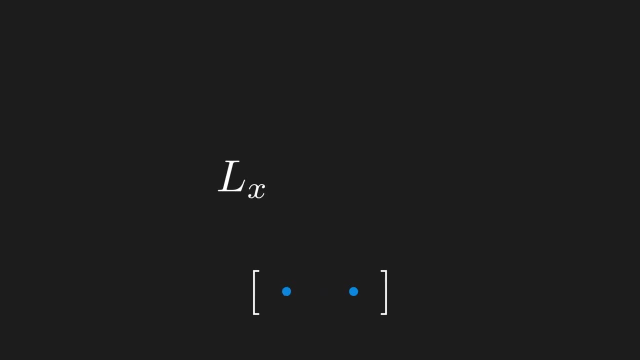 The first column tells us where the x basis vector goes. So plugging in, which has a component of 1 on the x axis, we get a 1 in the first column. The next column tells us where the y basis vector goes. 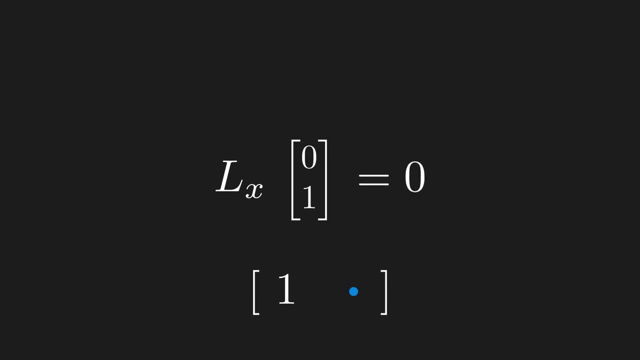 plugging in 0, 1, which has a component of 0 on the x-axis. We get a 0 here And this is the matrix of this linear functional. So we see that we get what's called a row matrix. 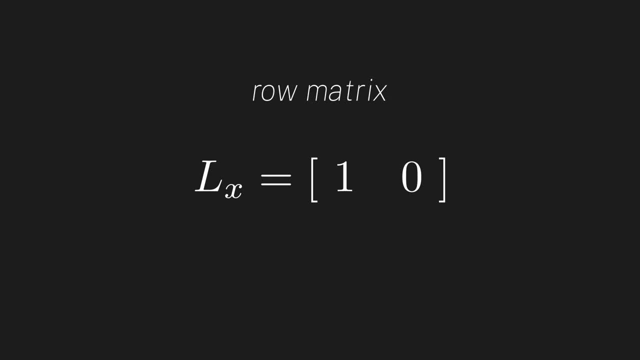 It's essentially a column vector on its side, and what it does is it takes in a column vector and spits out a number. Now let's take a step back. Remember that in R2, a linear functional is a linear map that takes us from two dimensions to one dimension. 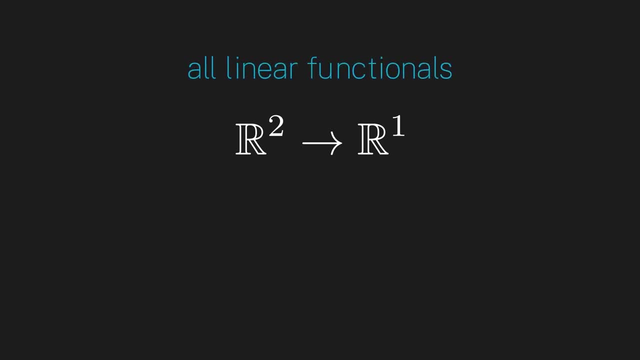 By definition, this means that all linear functionals in R2 are represented by 1, by 2 row matrices. So the set of all linear functionals in R2 consists of the set of all row matrices, Much like column vectors. this set of all row matrices. 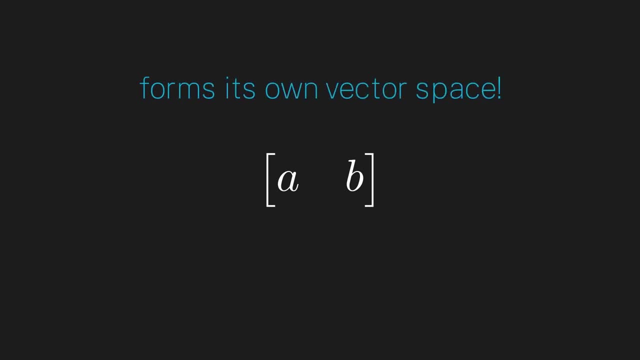 actually forms its own vector space, Seriously check all the conditions they work. This vector space is known as the dual space. Hopefully you see why it's called a dual space. Take your vector space of column vectors. turn them on their side. 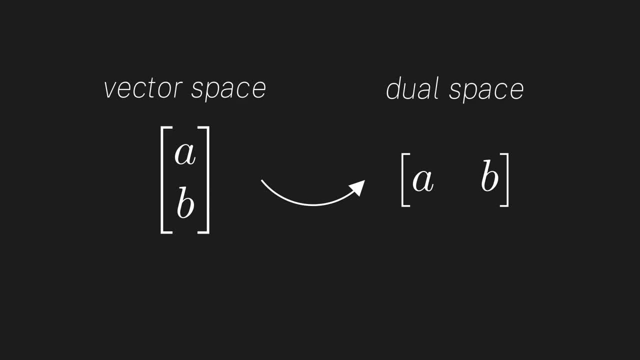 and what you get is the dual vector space of linear functionals. This has been specific to R2, but the dual space is a very useful concept in abstract vector spaces. Formally we define the dual space as follows: Given a vector space, V. 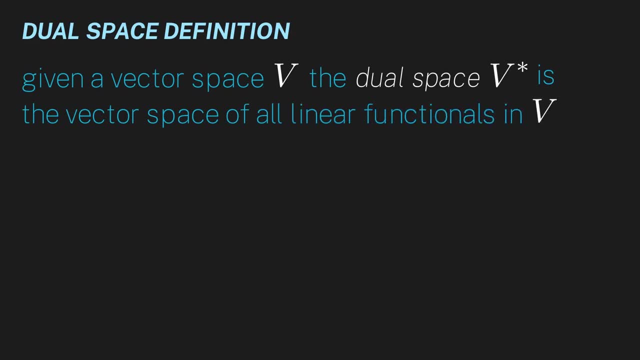 the dual space. V star is the vector space of all linear functionals in V which, remember, are just maps that take in vectors and spit out numbers. So all linear functionals L live in V star, Although this is an abstract definition. 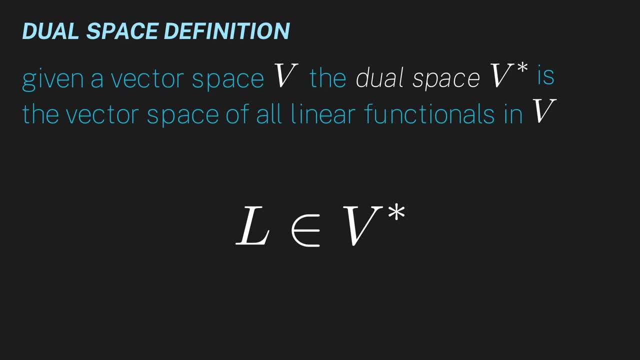 keep the intuition that the dual space is analogous to the space of row matrices. Now I remember when I first learned about functionals in the dual space. I thought it was unnecessary for quantum physics. But think about it. Our goal is to build a mathematical model. 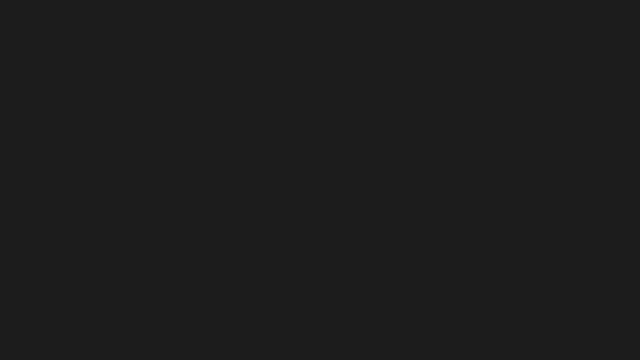 for the real world and in the end, we want to be able to extract values and predictions from it. For example, given our quantum state, say we want the probability of getting an energy of three electron volts. Or say we want the average position we expect in this state. 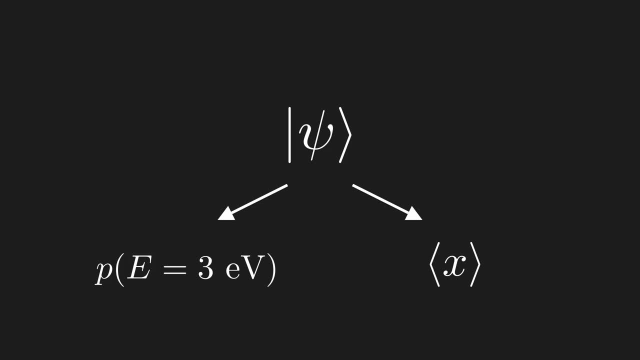 To get these we have to go from quantum state to number, and so we know that a linear functional is involved here somewhere. So hopefully you're convinced that we have to use linear functionals in our quantum theory. In fact, linear functionals are so important. 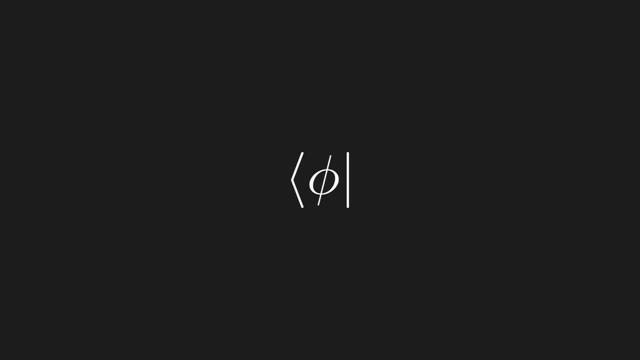 that we will ascribe a special symbol for them in quantum mechanics, a symbol called a bra, written as a backwards ket. Remember that this is a linear functional, so this should be seen as an operator that acts on a ket and returns a number, possibly complex. 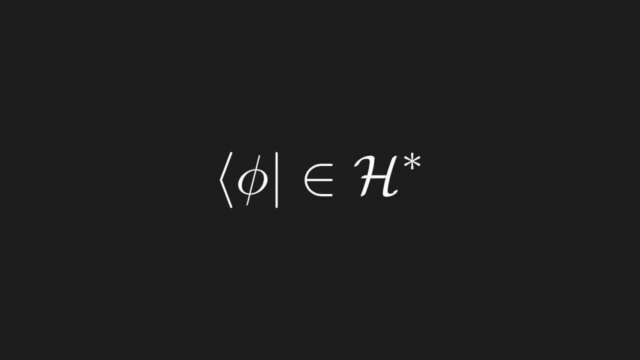 As we stated before, these bras live in the Hilbert dual space. That being said, you may be noticing something: When we put a bra and ket together to get a number, it looks suspiciously like an inner product in this notation. Yet we have made zero mention of the inner product. 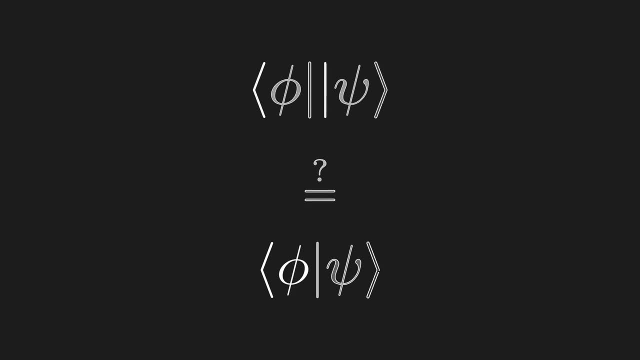 So what's going on? To begin solving this puzzle, let's go back to our LX operator in R2.. Take a second to notice how LX acts on a column vector. Do you notice how it is as though we are taking the dot product with the x unit vector? 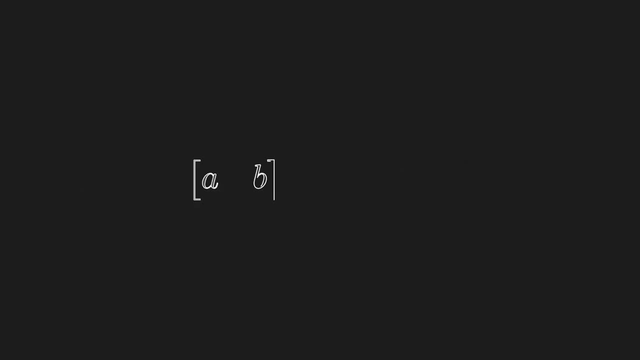 In fact, when a linear functional in R2 acts on any vector, it can be written equivalently as a dot product with the corresponding column vector. This is actually a very deep and general mathematical fact rooted within something called the Riesz representation theorem. 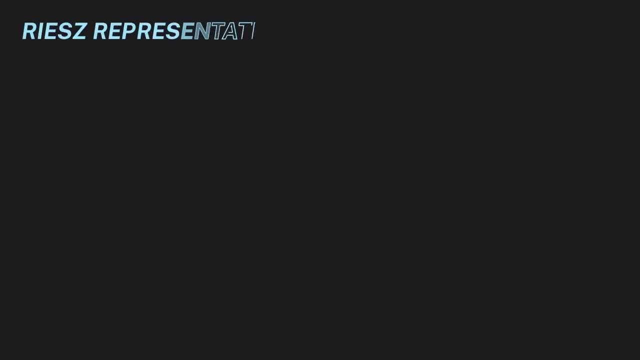 This sounds kind of daunting, but it's just a theorem about what we discussed. The theorem states that for any linear functional L phi, the action of L phi is a function of L phi. So let's take a look at this. Let's take a look at this. 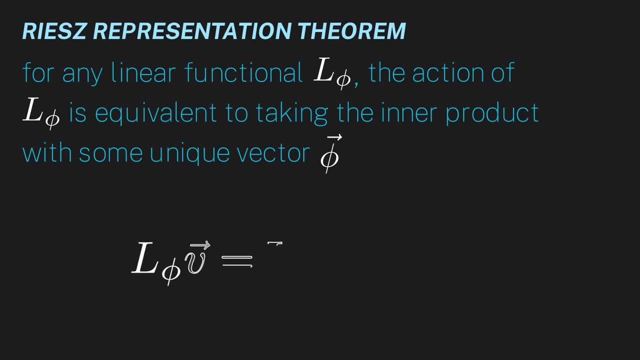 Let's take a look at this. This is equivalent to taking the inner product with some unique vector, phi. I won't prove the theorem here, but there are a slew of internet sources that have given rigorous proofs, if you're interested. So in our R2 example. 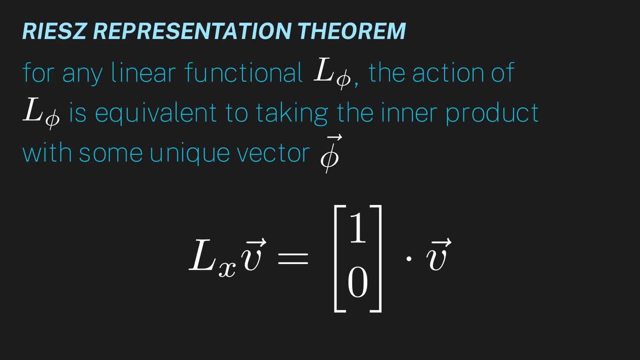 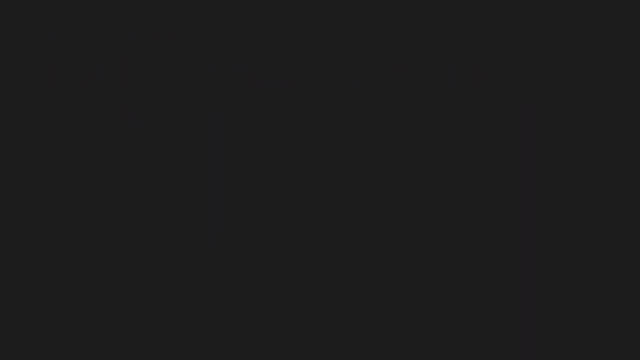 this unique vector was 1, 0, and acting with the LX operator was equivalent to taking the dot product with 1, 0.. And now, hopefully, you see why we chose our suggestive notation for a bra. A bra is just a flipped ket. 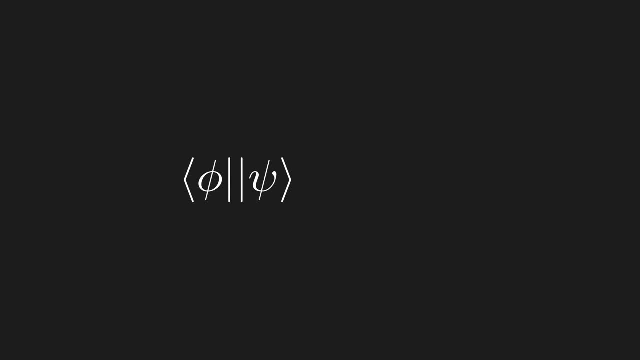 because the action of the dot product and the action of the bra linear functional is mathematically equivalent to taking the inner product with that ket. This notation for bras, kets and inner products is collectively known as Bra-ket notation or Dirac notation. 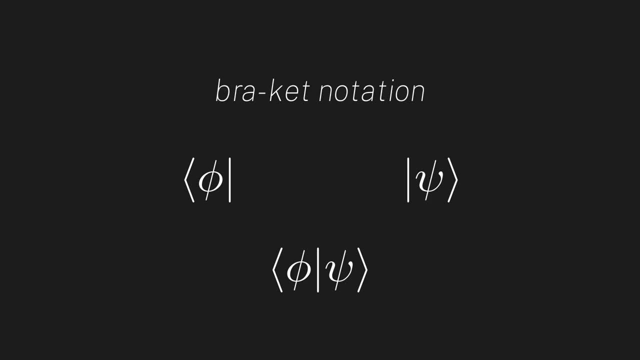 as he was the first to use it in quantum mechanics. So why is this notation so powerful? As you can see, it has the Riesz representation theorem baked right into it. You can break apart inner products and put together bras and kets. 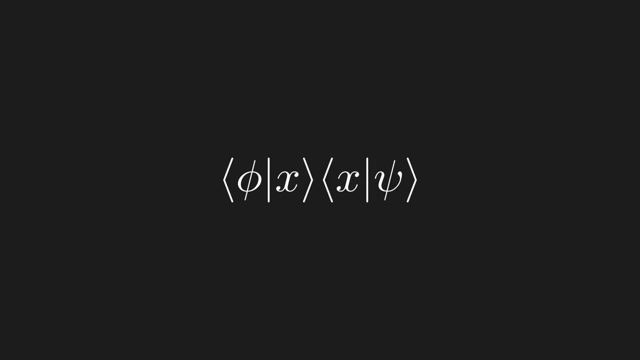 however you please, and you can be rest assured that whatever you get still makes mathematical sense, all because of the Riesz representation theorem. I mean, really think about this: Although a bra and the inner product are formally completely different mathematical entities, Bra-ket notation makes their connection absolutely seamless. 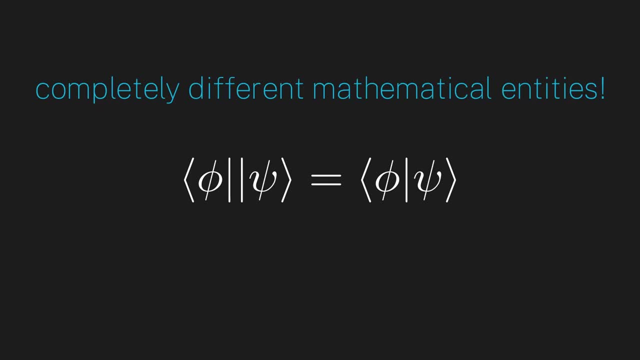 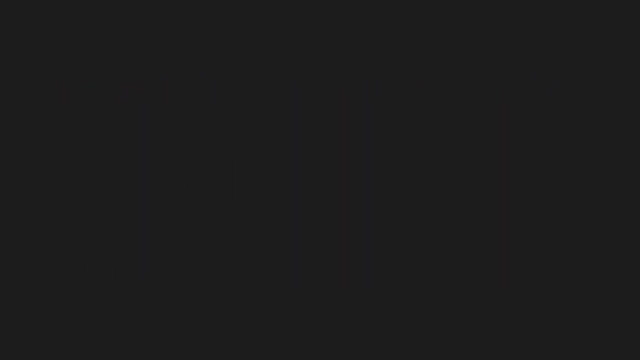 Let Bra-ket notation do all the work. To really show you the power of Bra-ket notation, I want to run through a quick example. Let's say we have an orthonormal basis in our vector space and we expand an arbitrary quantum state. 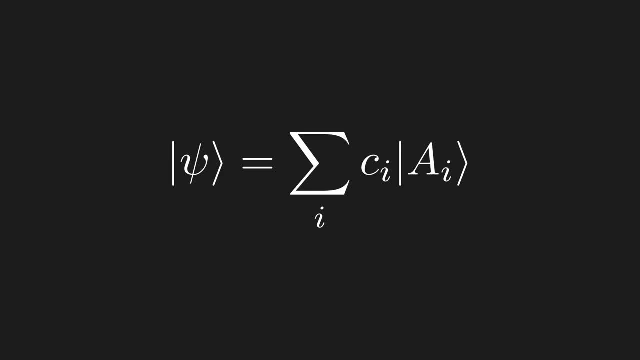 in this orthonormal basis. Remember from chapter four that because all the states are orthonormal, we can calculate the coefficients as follows. It's also really easy to prove this yourself, So let's plug in this expression: for all the coefficients.